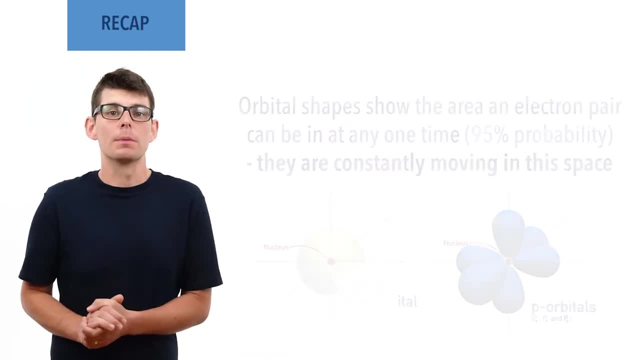 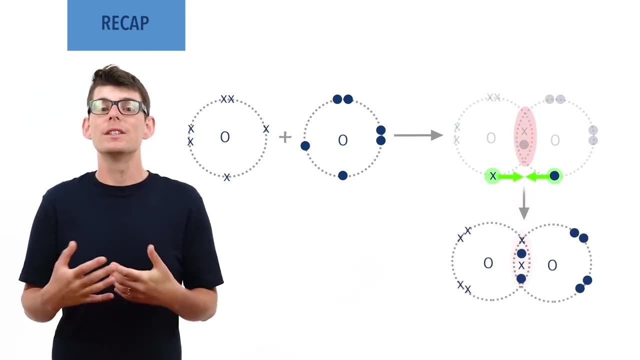 Other half-filled atomic orbitals can sometimes also overlap or merge, creating another bonding orbital between the two atoms, leading to a double bond. The atoms are harder to split apart when double bonded together, although the second bond is weaker than the first single bond. 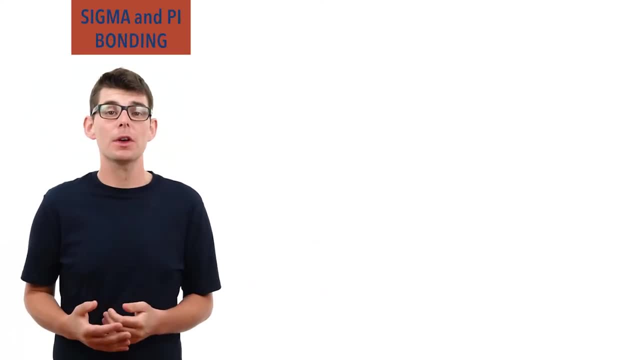 Recap done, let's go As mentioned. to form a covalent bond between two atoms, atomic orbitals must overlap or merge to create a bonding orbital. The two atomic orbitals face each other and if the orbitals can overlap easily, the bond. 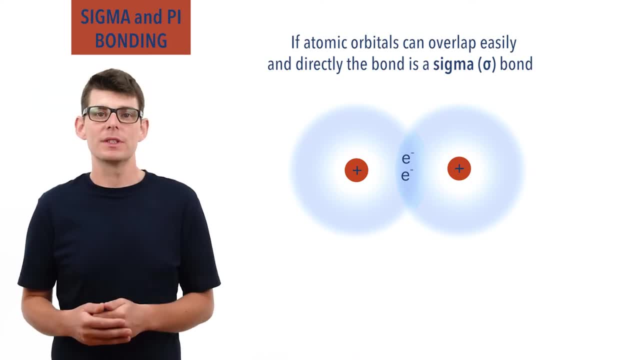 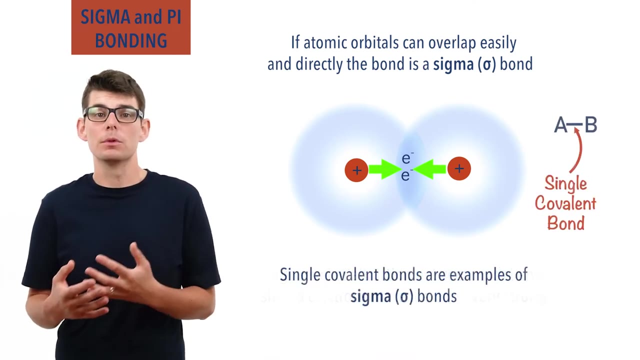 formed is called a sigma bond, shown with the Greek symbol for sigma. The bonding orbital is close to the nuclei of both atoms and the nuclei. both have a high level of attraction to the electrons in the orbital, making the bond very strong. Single bonds are always examples of sigma bonds, as atoms will always try and arrange. 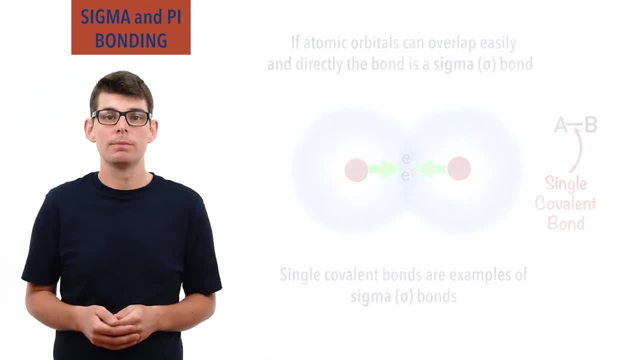 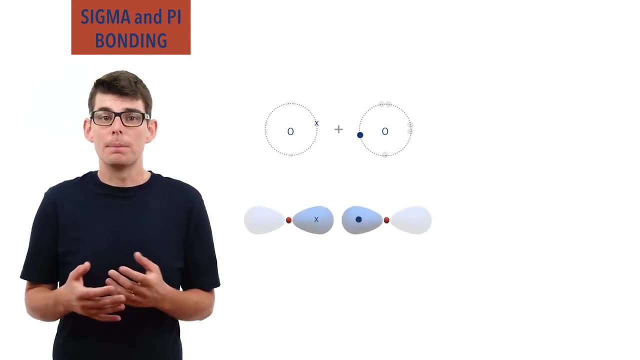 themselves to maximise the overlap of two orbitals, For example in an oxygen molecule. each oxygen atom has a half-filled p-shaped orbital. The p-shaped orbitals have lobes that stick out of each side of the nucleus and the lobe. 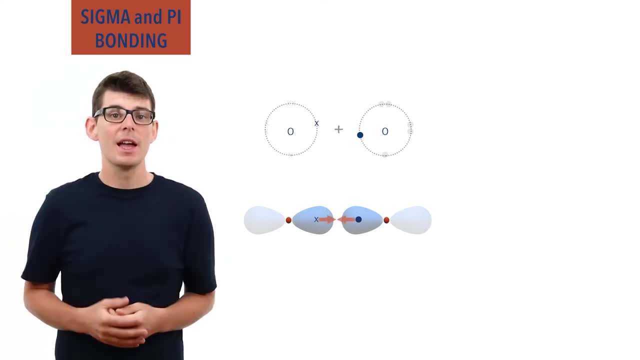 from each p-orbital, from each atom can point towards each other and the two can overlap and merge. The bond formed is a sigma bond, as the both orbitals overlap directly. The bond is also free to rotate, as rotating each nuclei has no impact on the bond. 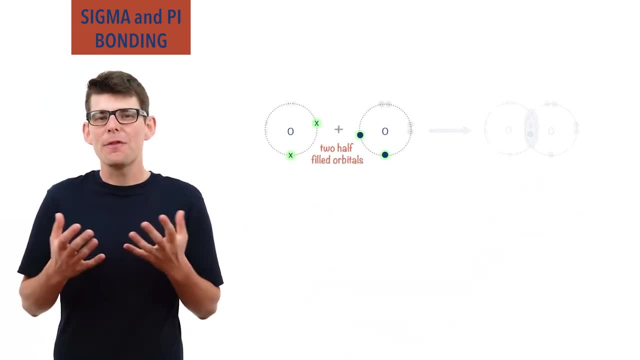 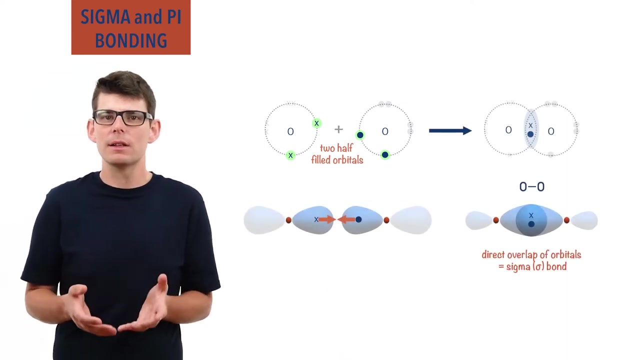 Before the oxygen atoms formed a sigma bond, they each had two half-filled p-orbitals. The sigma bond was formed from the direct overlap of one of these from each atom. This means that each oxygen atom still has a half-filled p-orbital and wants to form 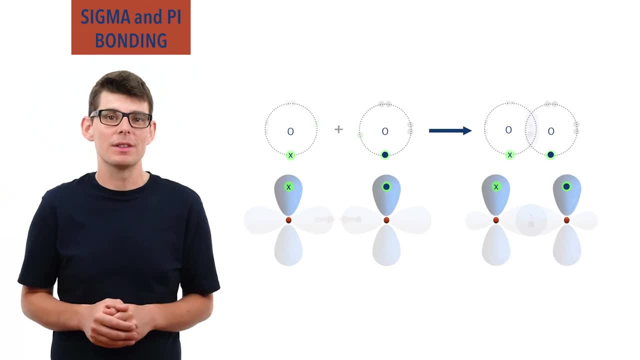 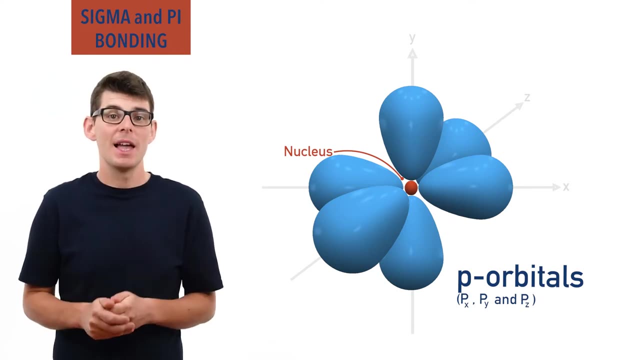 another bond. Now things can get a bit interesting. Remember that there are three p-shaped orbitals around the nucleus: Px, Py and Pz. Px, Py and Pz- And their lobes are each pointing in different directions, all 90 degrees to each other. 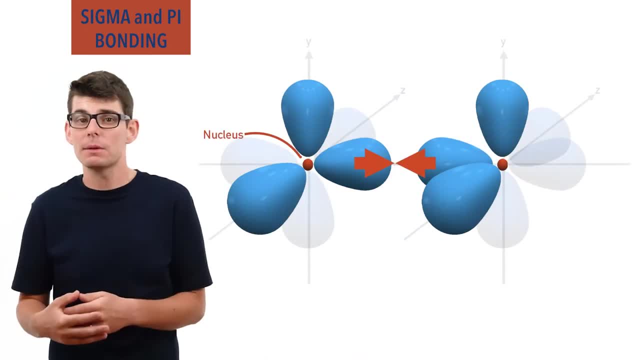 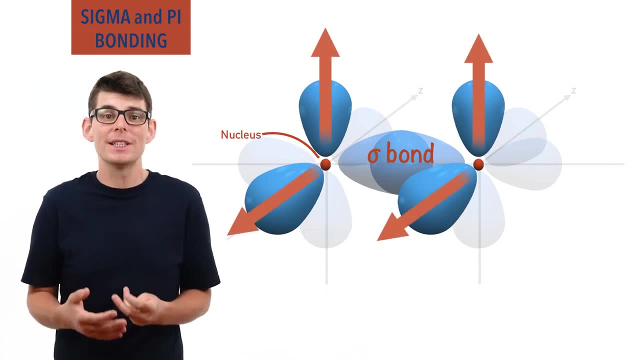 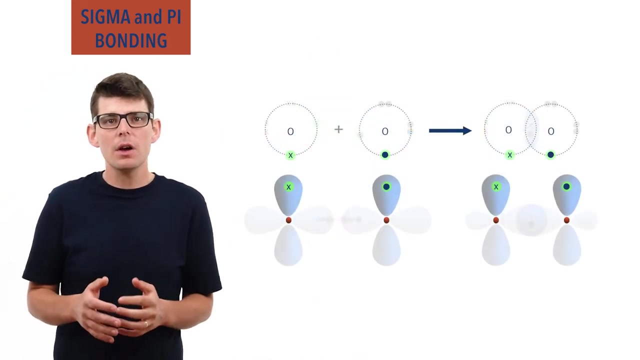 If two half-filled p-orbitals overlap fully to form a sigma bond, the half-filled orbitals left over cannot directly line up or overlap. They are simply pointing in the wrong direction. As the atoms are now quite close together due to the single sigma bond, the other half-filled 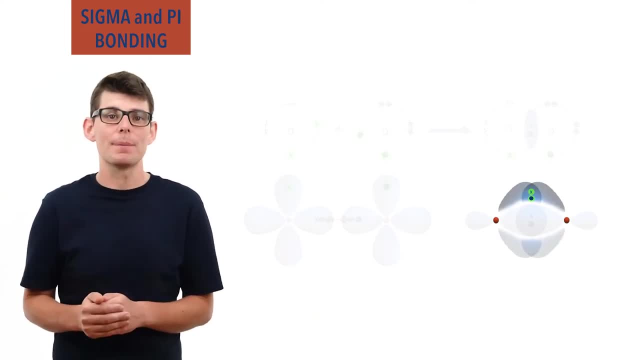 orbitals can actually bend inward slightly and overlap sideways. The electrons in this orbital are further from the nuclei of both atoms compared to the sigma bond, and the bond is therefore weaker. This type of bond is called a Py-bond, shown with the Greek symbol Pi. 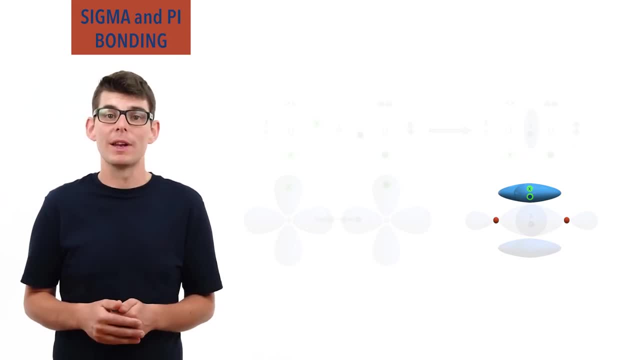 Due to each orbital having two lobes, the p-orbitals overlap sideways, creating two areas of electron density above and below the sigma bond already formed. This means the bond is now unalienable. This means that the p-orbitals overlap sideways, creating two areas of electron density above. and below the sigma bond. This means that the p-orbitals are unable to rotate freely. If one atom rotates, the p-bond in orbitals will try to rotate as well, meaning they'll become twisted and if twisted too far, will break. 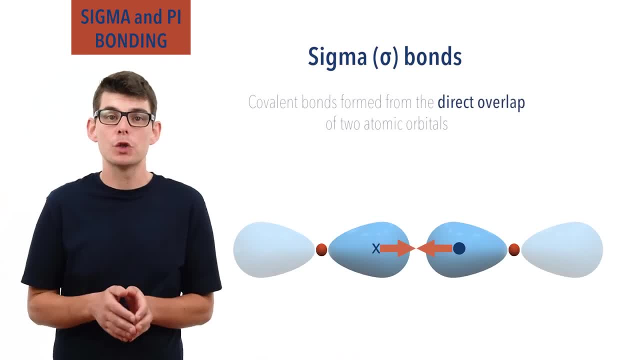 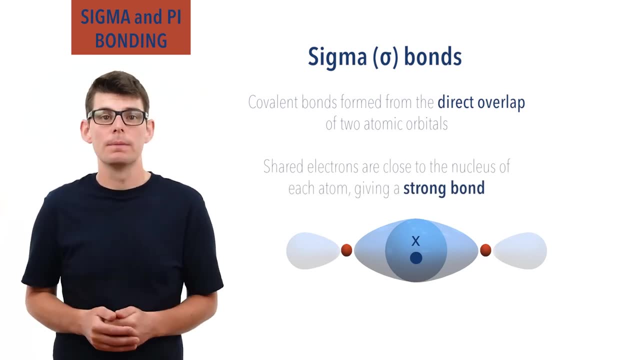 Sigma bonds are covalent bonds that form from the direct overlap of two orbitals from two atoms. Electrons in the bond are close to the nuclei of both atoms and the bond is strong. Pi bonds are covalent bonds that form from the sideways overlap of two p-shaped orbitals. 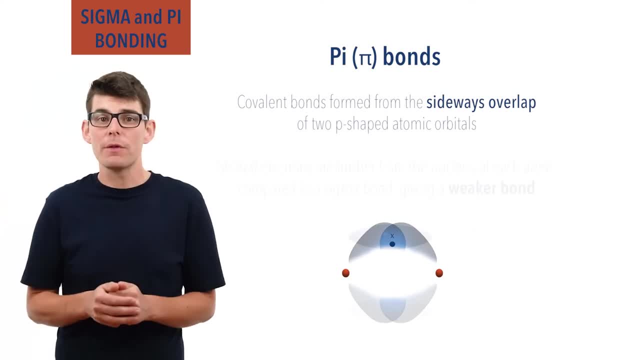 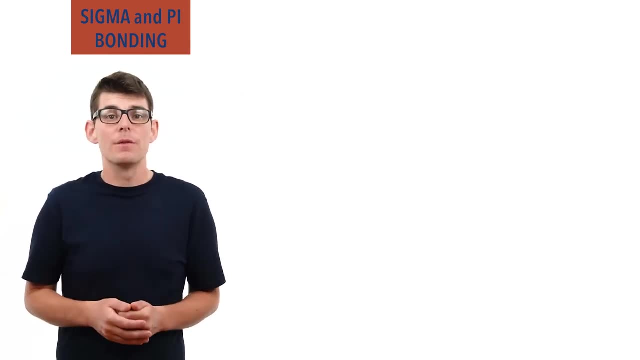 from two atoms. Electrons in the bond are further from the nuclei of both atoms and, as a result, pi bonds are weaker than sigma bonds At this level. the carbon bonding in ethane and ethene is often used to model sigma and 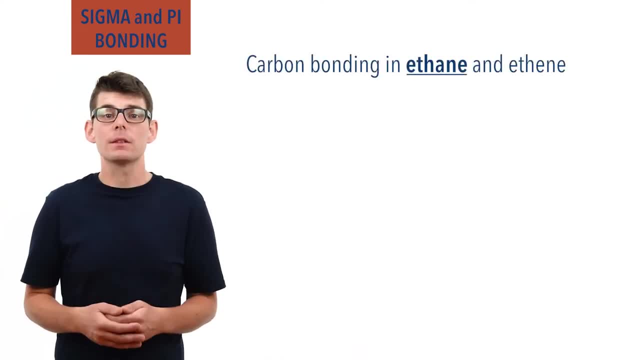 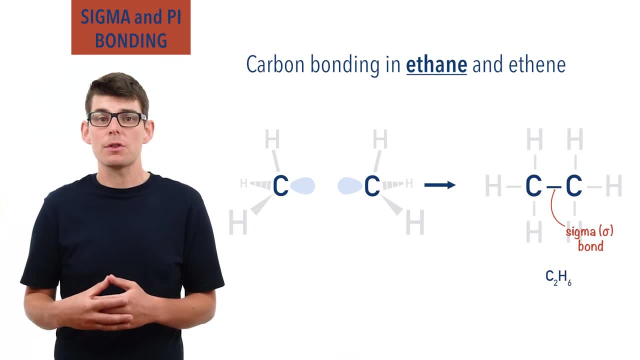 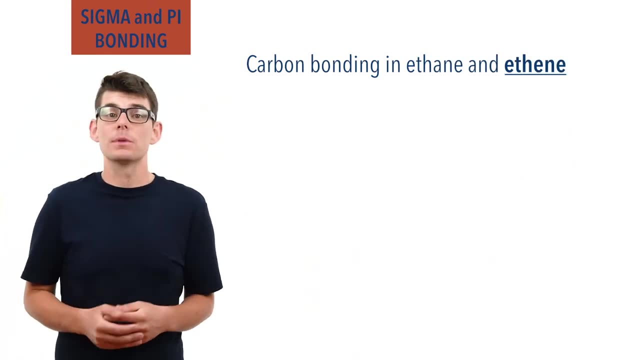 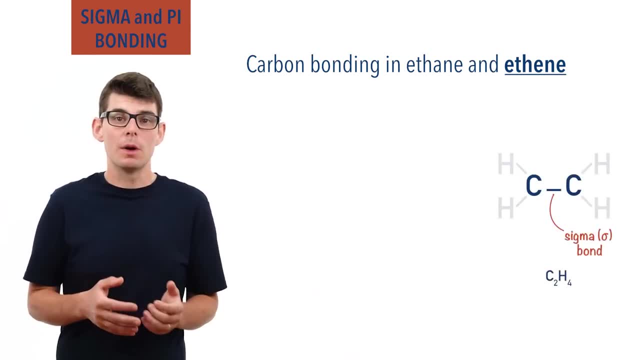 bond, as well as the sideways overlap of two other orbitals, a pi bond. This is referred to as a carbon-carbon double bond. Each carbon atom has two bonds to hydrogen atoms, and this leaves two half-filled p-shaped orbitals left over. 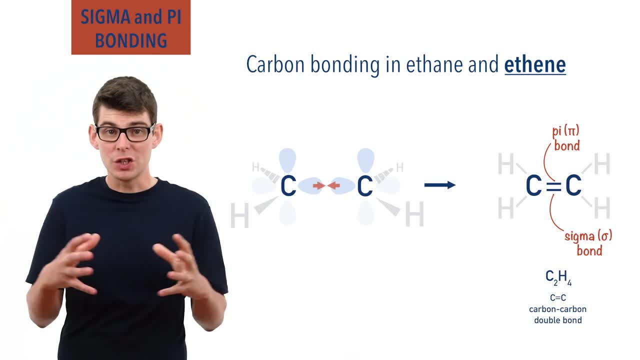 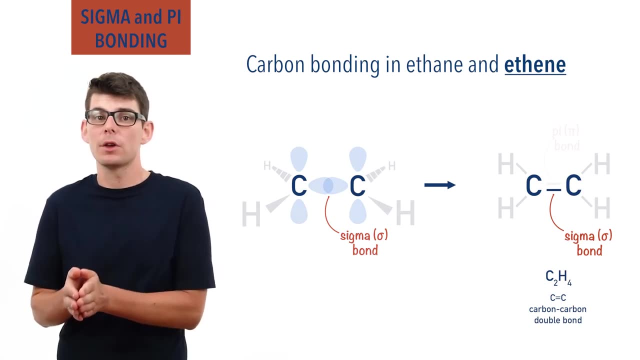 To start with, the carbon atoms will arrange themselves to have that direct overlap of two orbitals and a sigma bond will form. This will leave two p-shaped orbitals left over that can overlap sideways between the two atoms, forming a pi bond. There are now essentially two bonds between the carbon atoms: a sigma bond and a pi bond. 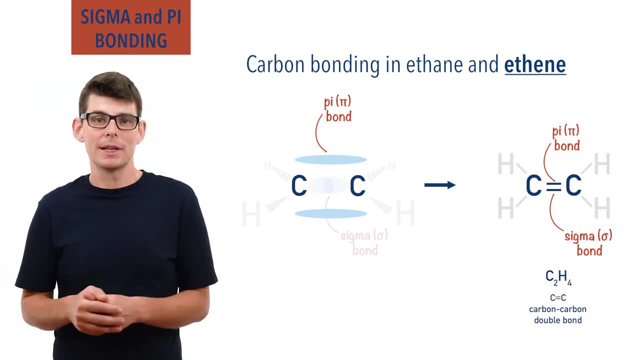 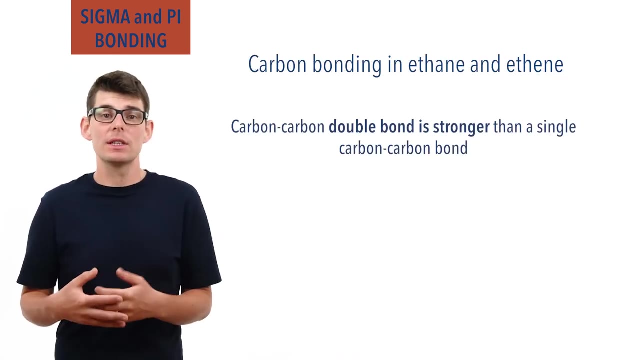 This is called a double bond and is shown as two lines between the carbon atoms. One line represents the sigma bond and the other the pi bond. As the carbon atoms are held by two bonds, a carbon-carbon double bond is stronger and harder to break than a single carbon bond. 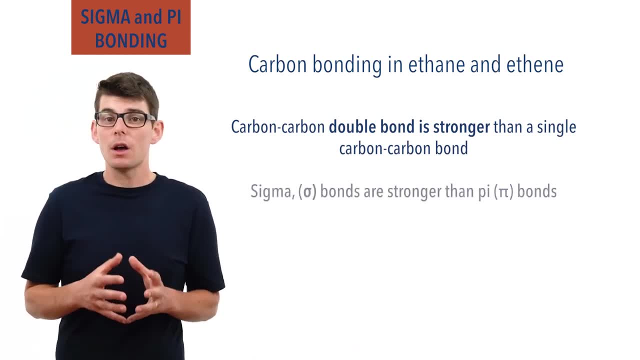 Sigma bonds are stronger than pi bonds, however, meaning that a carbon-carbon double bond isn't twice as strong as a carbon-carbon single bond. It is easier to break a pi bond than a sigma bond. This actually gives ethene a higher range of carbon-carbon double bonds. 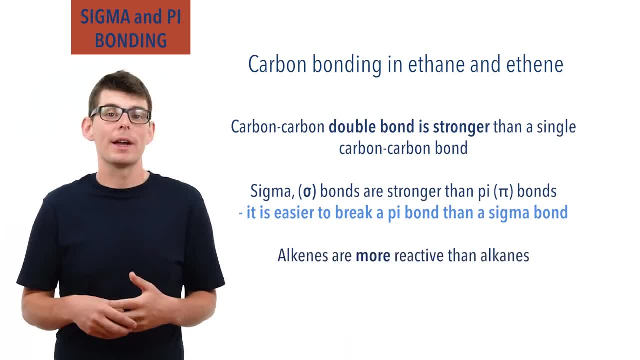 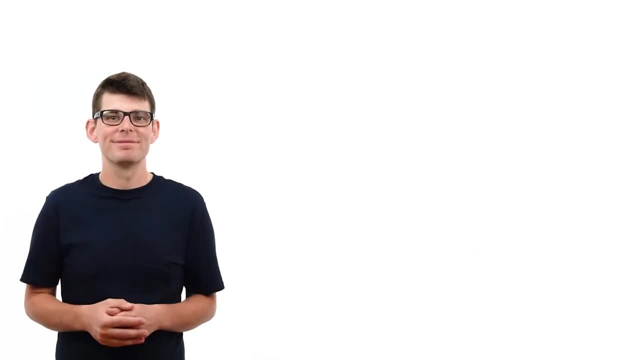 It has more reactivity than ethane and explains why alkenes are more reactive than alkanes. If a pi bond is broken, the sigma bond between the atoms still remains. So, to summarise, covalent bonds are formed from the overlap of two atomic orbitals from two atoms. 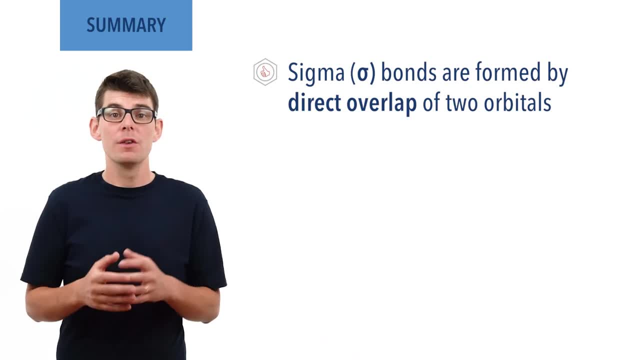 Sigma bonds form from the direct overlap of atomic orbitals from two atoms. Electrons in the bond are close to the nuclei of both atoms, giving a high level of attraction that is hard to break, making sigma bonds strong. Sigma bonds are free to rotate. 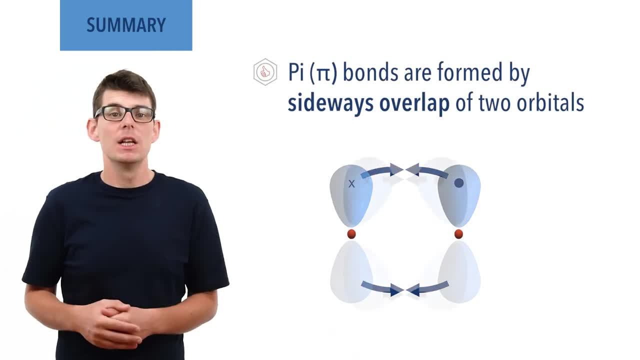 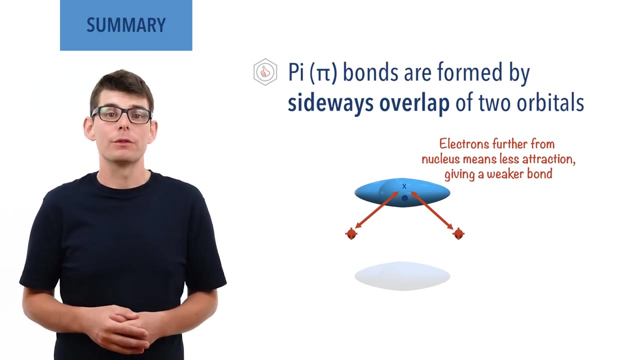 Pi bonds form from the sideways overlap or bending of p-shaped atomic orbitals from two atoms. Electrons in the bond are further from the nuclei of both atoms compared to a sigma bond, giving weaker attraction and a bond that is easier to break. As p-shaped orbitals have two lobes, a pi bond has two areas of electron density. 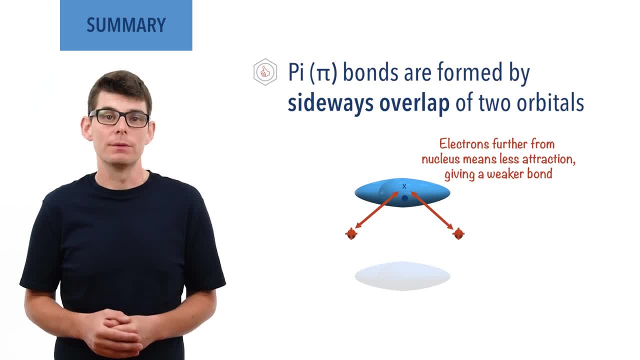 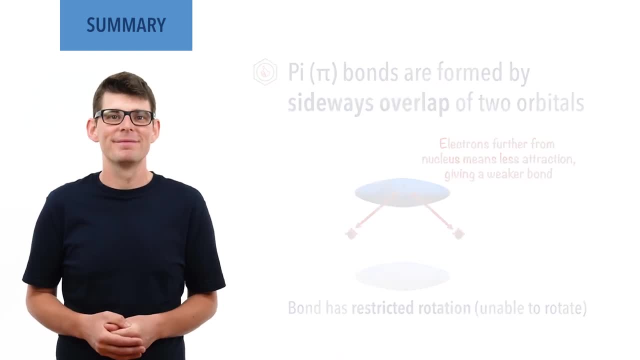 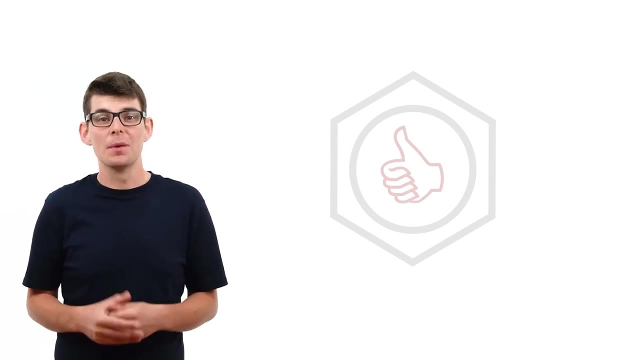 one above and one below a sigma bond already found. There is restricted rotation and the pi bond is unable to freely rotate and twist. I hope you found this video useful. please check out other relevant videos in the links given in the description below and visit chemistrystudentcom for free notes and revision materials.